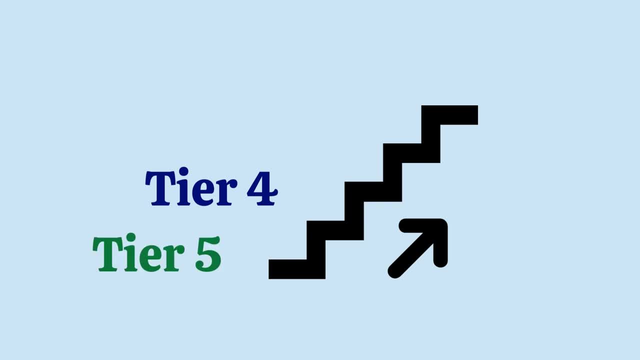 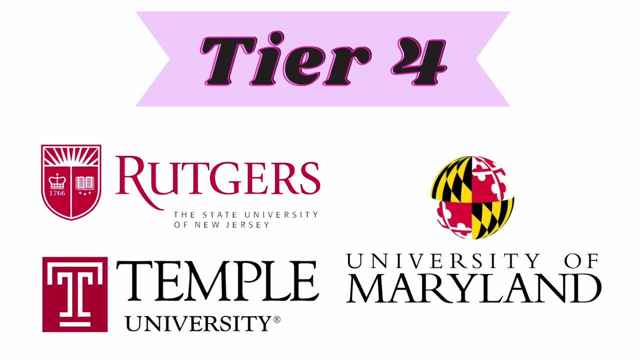 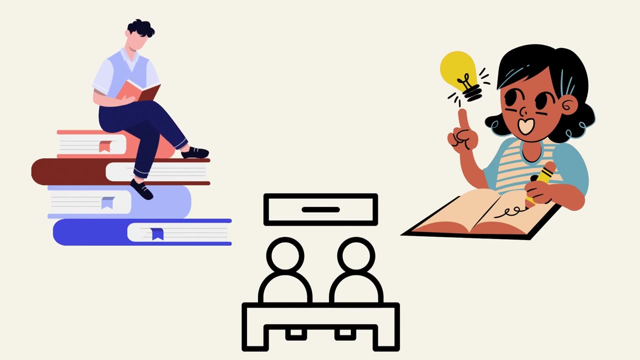 up in. It's a bit harder to get into these schools than tier 5 schools. Schools in this tier include Rutgers, Temple University and University of Maryland, College Park, Tier 3.. Students in this tier probably tried a lot more in high school than students in tier 4. 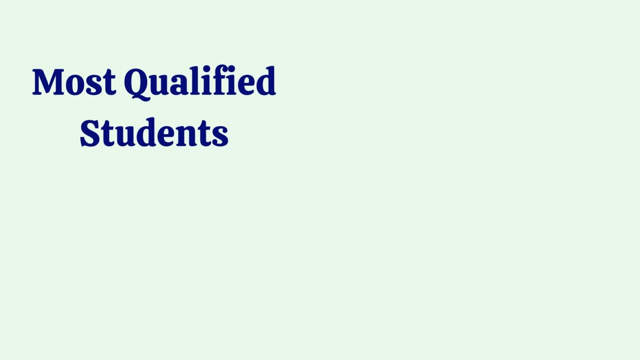 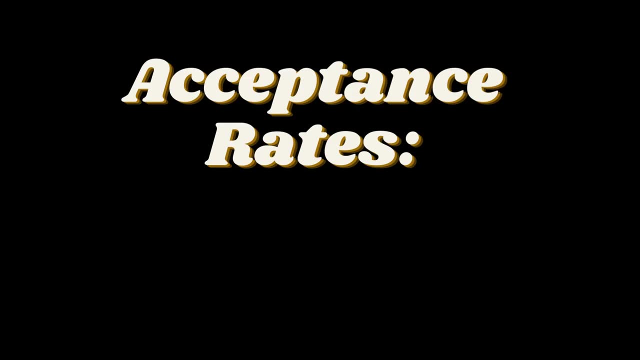 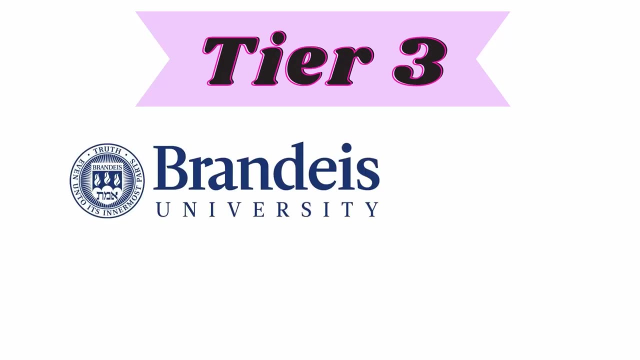 and 5. The most qualified students will be able to treat these as safety schools, while less competitive candidates should treat them as targets. Acceptance rate is a bit higher in high school than in tier 4 and 5.. The rates for these schools are around 35%. Tier 3 schools include Brandeis University. 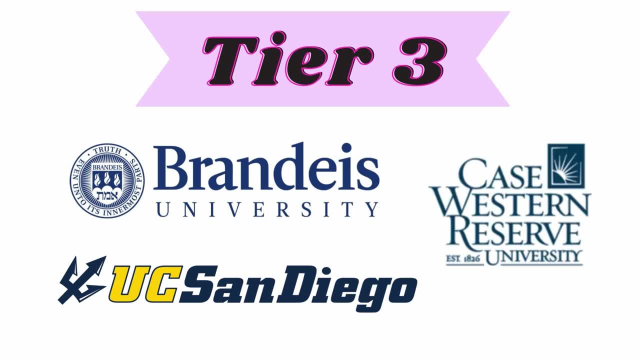 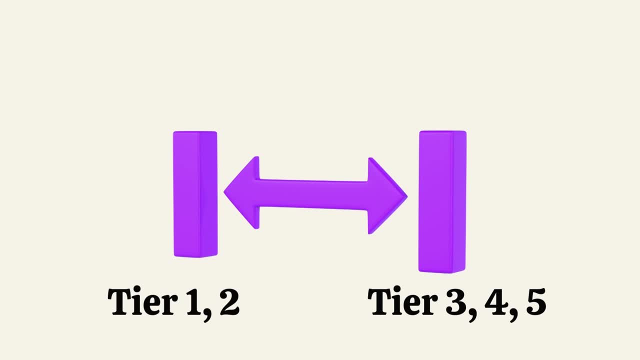 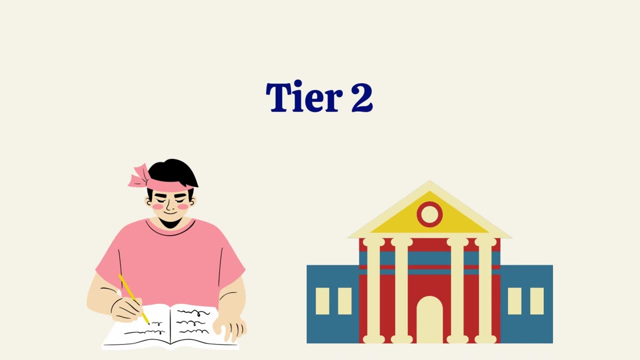 UC San Diego and Case Western Reserve University, Tier 2.. There is a big gap between the last three tiers and tier 1 and 2 in terms of academics and personal ambition and goals. These schools are quite competitive and harder to get into than. 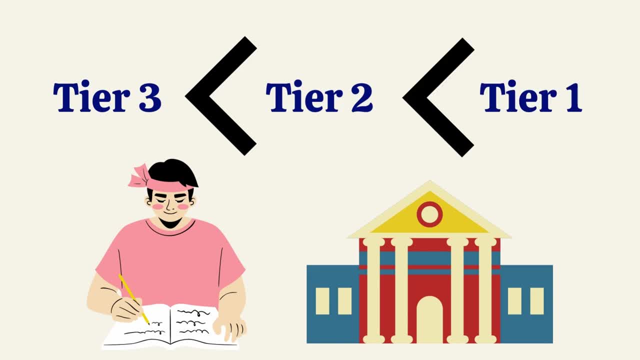 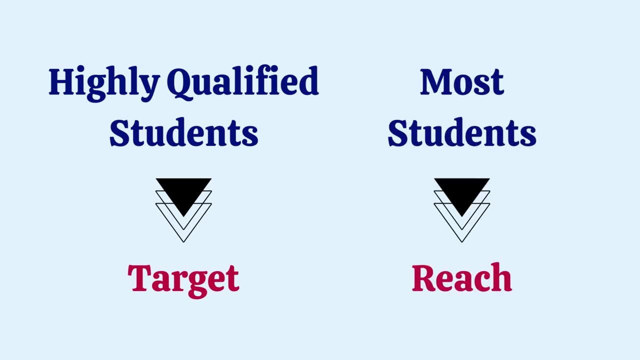 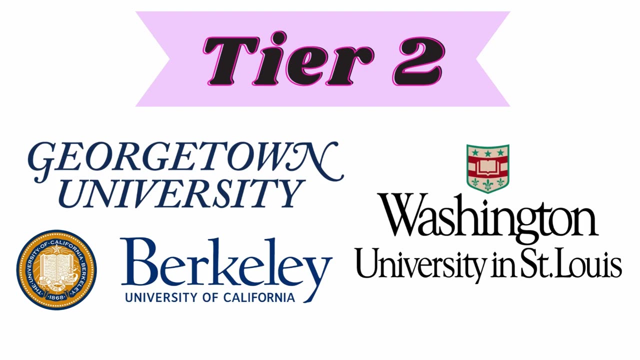 tier 3 schools, but less so than tier 1.. Highly qualified students may count these schools as target and most students can count them as reach schools. Tier 2 schools include Georgetown, UC, Berkeley and Washington University in St Louis. 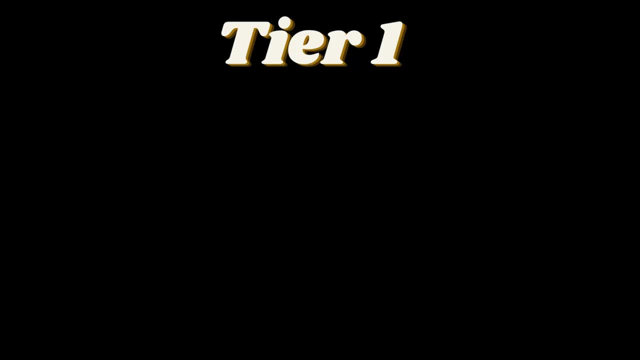 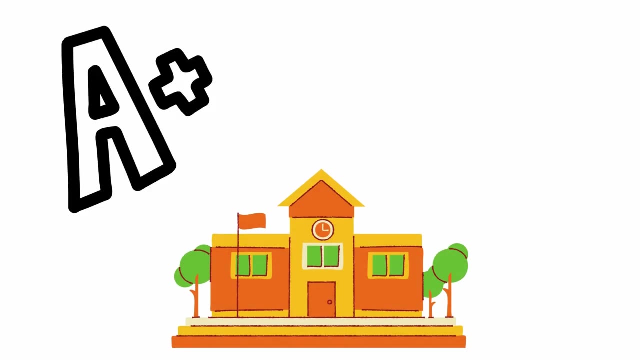 Tier 1.. Finally, tier 1 includes the famous schools where students with high ambitions and perfect scores go to. These schools want academic excellence and stellar extracurriculars, but those are not the case. Tier 1 schools are more likely to get into these schools than tier 1.. 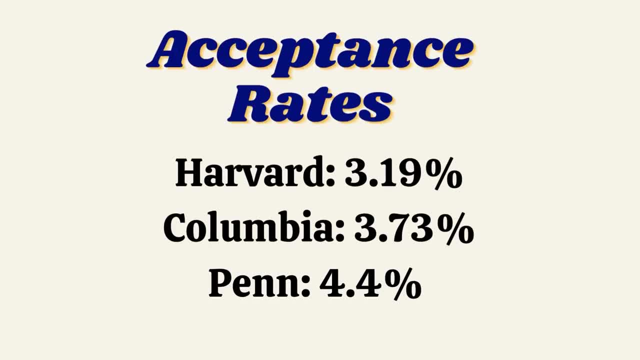 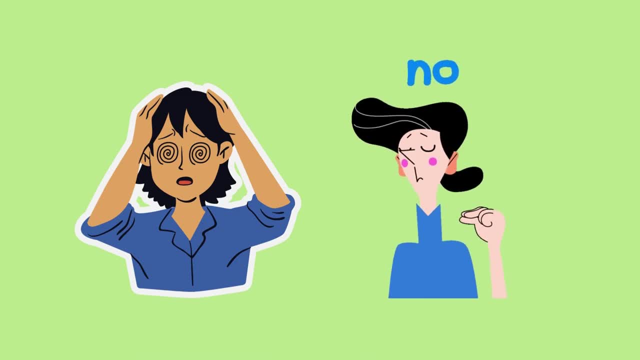 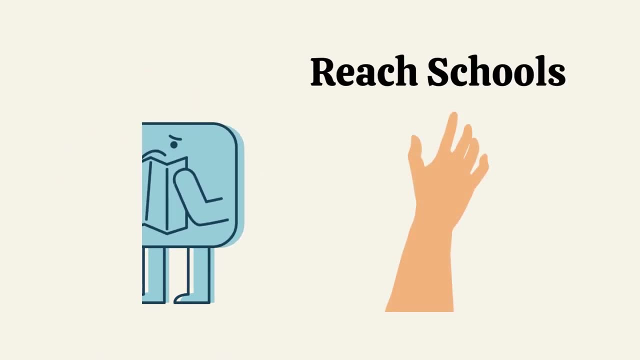 Not enough to get you in. With acceptance rate as low as 3%, getting accepted isn't impossible, but it should never be treated as guaranteed. These are the most difficult schools to get into and will be reach schools for even the most qualified students. 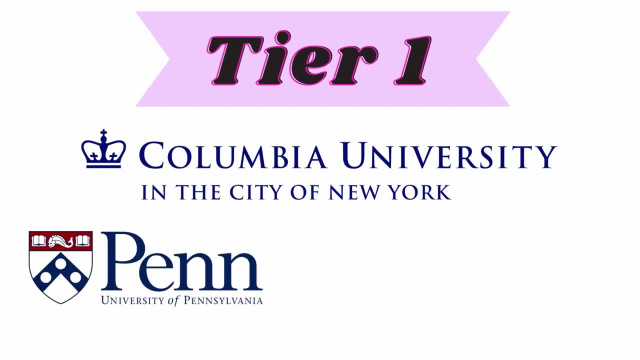 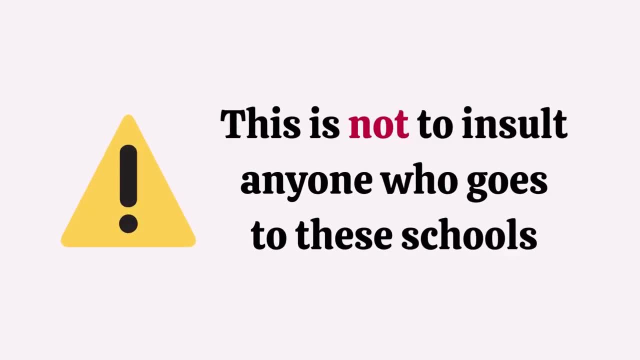 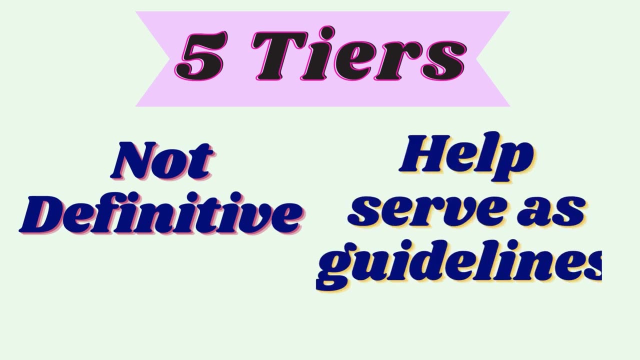 Schools in this tier include Columbia, UPenn and, of course, Harvard. That's the five tiers of colleges in the United States. This is not to insult anyone who goes to these schools. These tiers aren't meant to be definitive, but rather help serve as guidelines when picking. 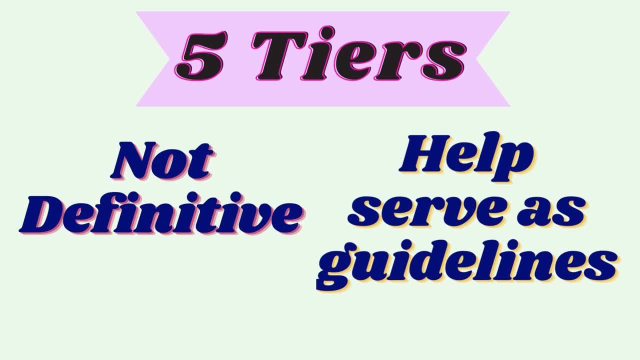 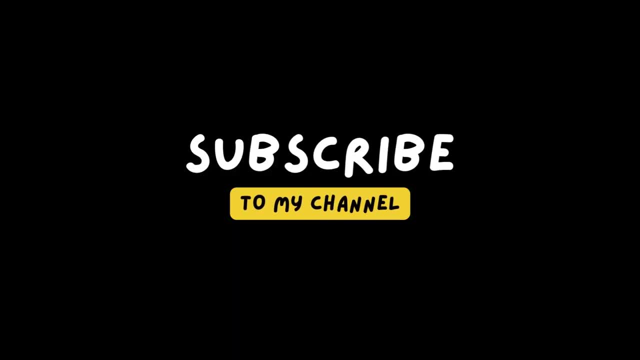 which schools you want to apply to and determining which schools you have the best chance of getting accepted to. Thanks for watching and please like and subscribe for more interesting videos. Bye.